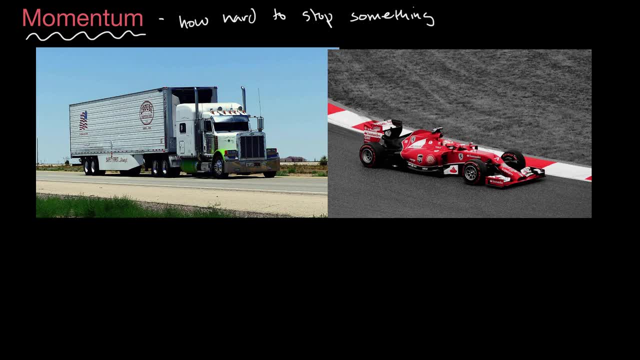 and here we have a Formula One car. Let's say that they both have a velocity of 20 meters per second, positive 20 meters per second. We'll just think in one dimension. So let's say it's going to the right at 20 meters per second. 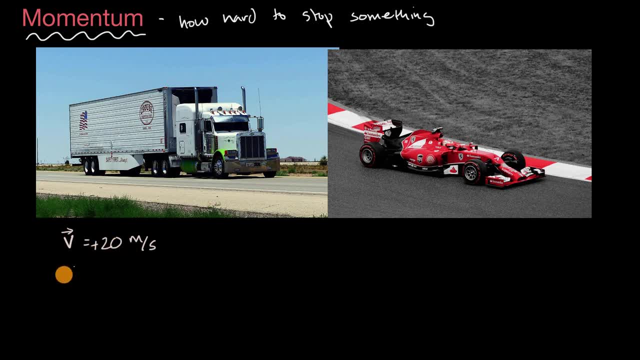 So that's a magnitude and a direction. Okay, I've got a positive here to make it clear that I'm giving a direction here. So they're both going in the positive direction at 20 meters per second, But you can imagine their masses are very different. 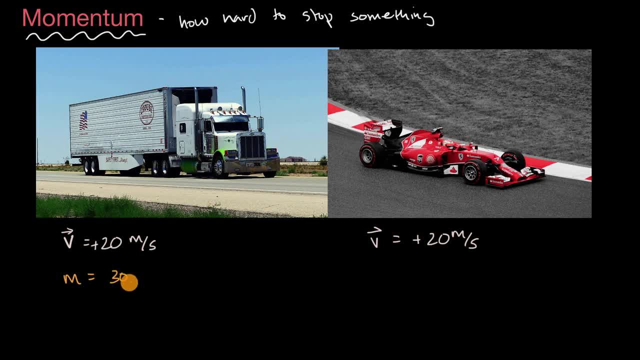 This large truck would have a mass of, let's just say, 30,000 kilograms. That's roughly actually what an 18-wheeler truck's mass is. I looked it up before this video And let's say the mass of this Formula One car. 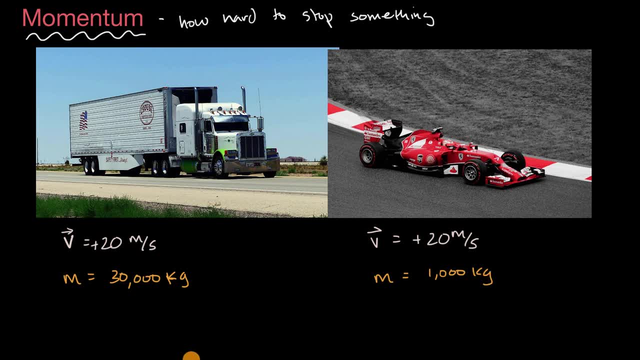 is about 1,000 kilograms. Now pause this video and think about which one do you think would have more momentum. All right, You're probably imagining trying to stop either of these, And I guess either of these would be difficult to stop. 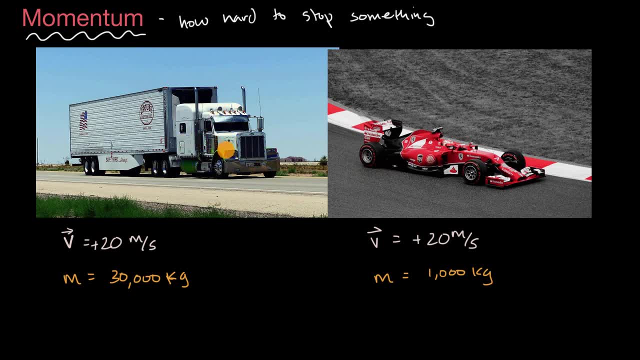 but a truck going at 20 meters per second seems a lot harder than the Formula One car. This thing seems like it would just be able to drive through anything. So if you picked the truck having a higher momentum when it's going at the same velocity as a Formula One car, 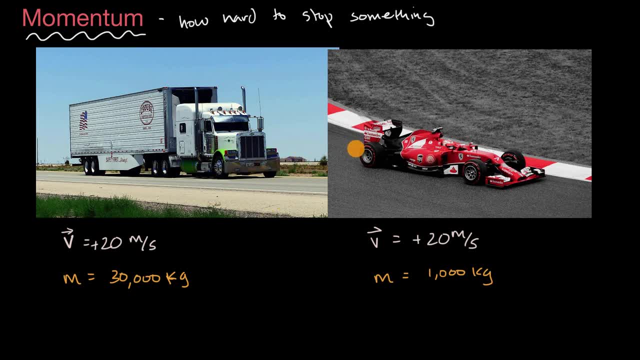 you'd be right. But an interesting question is: well, how can I quantify that? And that's where we have the mathematical definition of momentum. And momentum is defined as mass times, velocity, And because velocity is a vector, it's not just a magnitude, we assign a direction. 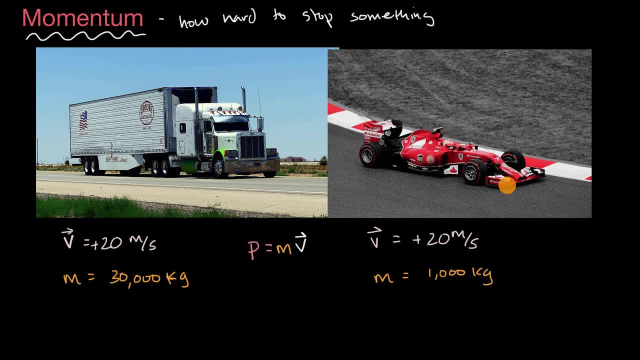 So we set it in the positive direction. If we were in one dimension, if we set it in the negative direction, we'd be going to the left. That's maybe the convention we could use And since it's a scalar which is mass times a vector, 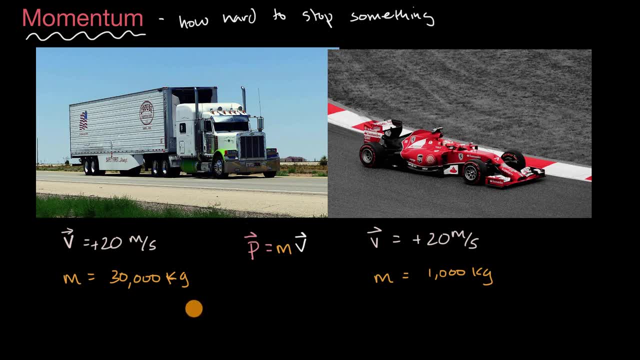 momentum is also going to be a vector. You're going to have a momentum in a certain direction. So pause this video and see if you can calculate the momentum for each of these vehicles And see also if you can figure out what the units are going to be. 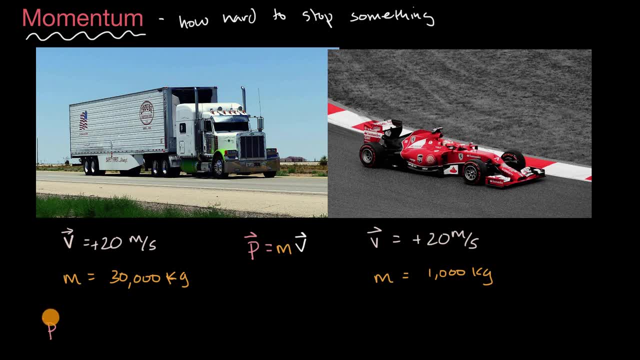 All right, now let's think about the momentum for this 18-wheeler. It is going to be its mass, which is 30,000 kilograms, times its velocity, which is positive 20 meters per second. And so when I multiply those two things, I am going to get 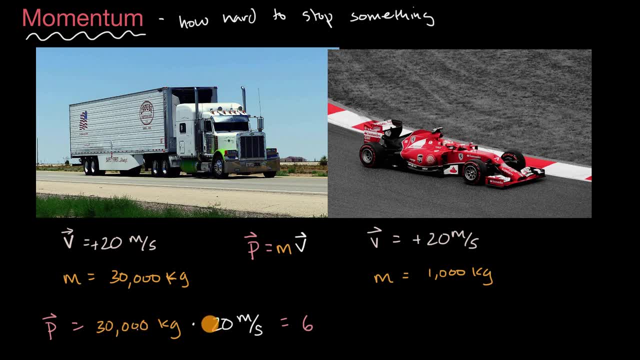 let's see, I'm going to get a six with one, two, three, four, five zeros. one, two, three, four, five zeros, 600,000.. And then the units are kilogram times, meter per second. 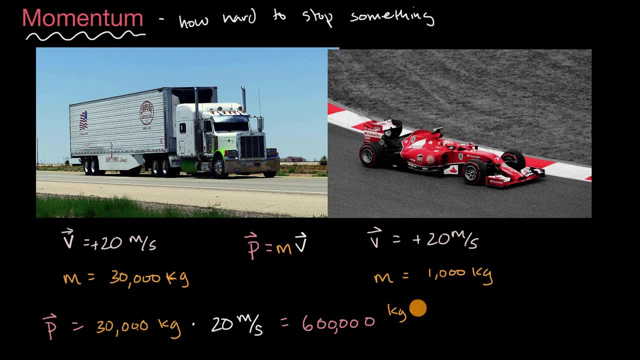 Kilogram meter per second. That's the momentum of the truck. Now what about the Formula One car? Pause the video and try to calculate that momentum. All right, well, same notion. I'll have to squeeze it in right over here. 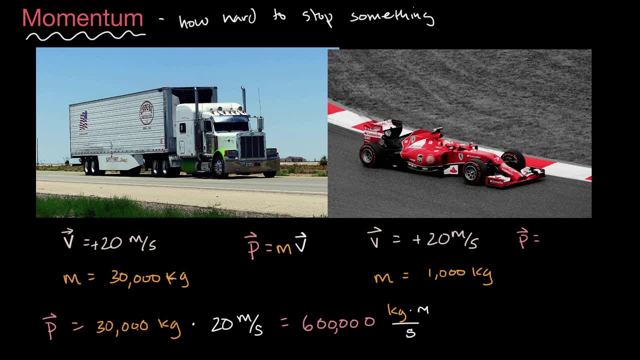 The momentum here is the mass: 1,000 kilograms. 1,000 kilograms times the velocity, positive 20 meters per second. I'm stressing the positive because we're in one dimension and I'm saying positive is one direction, negative is the other direction. 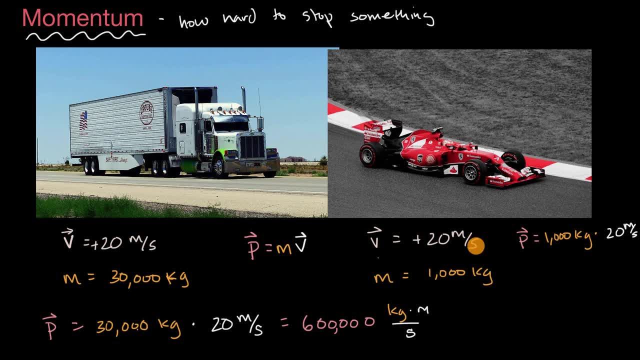 So I am giving a direction here, And so this momentum is going to be equal to 20,000 kilogram meters per second. Kilogram meters per second. And so when you evaluate the momentums, it's clear mathematically that the truck 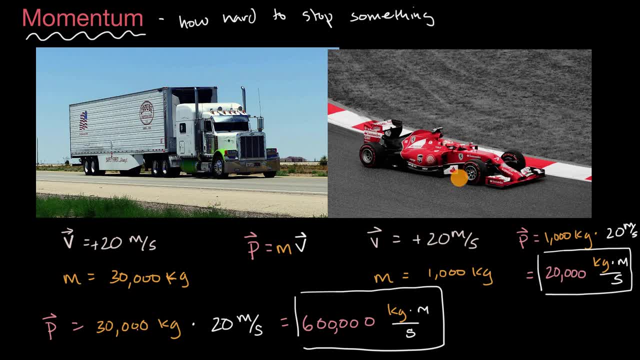 has much more momentum than this Formula One car. It has 30 times the momentum. Now I know what some of y'all are thinking. Well, this is just from the reference frame if I'm standing still on the ground while this truck and car are moving by. 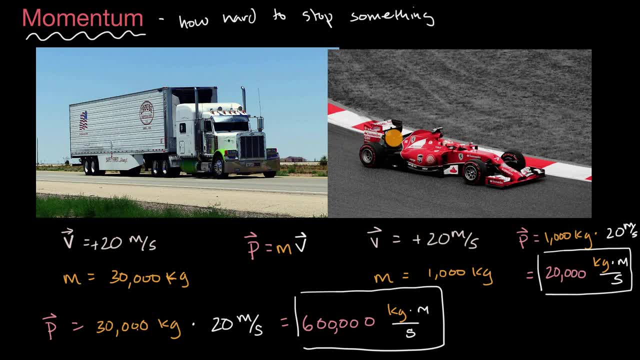 But what if I were moving along with them? Would they have the same momentum? And if you were asking that question, it's a very good one- And the answer is no. the momentum depends on the frame of reference. So let's say that you are able to travel very quickly in. 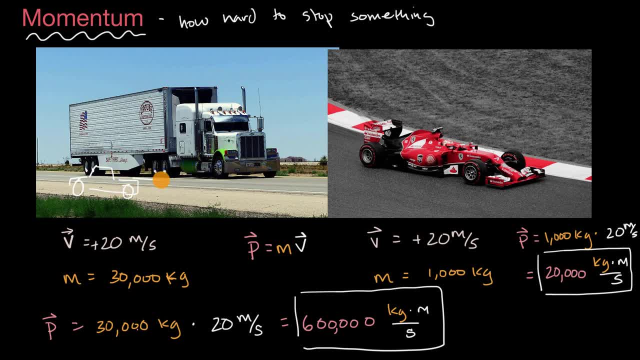 well, let's say you're in a car here and you're also going at 20, positive 20 meters per second. So you're going in the same direction as the truck. Well, relative to you, the truck's velocity is now zero.